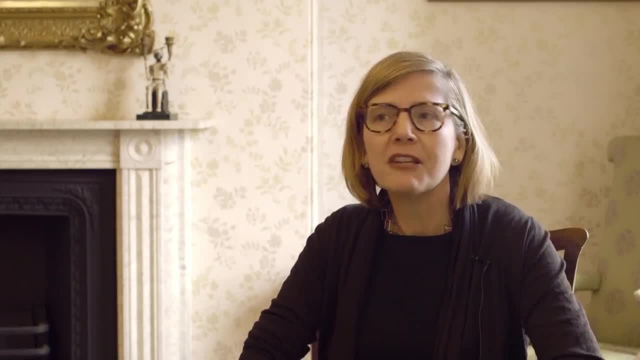 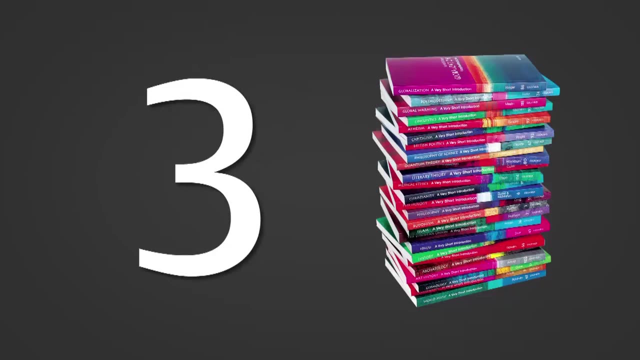 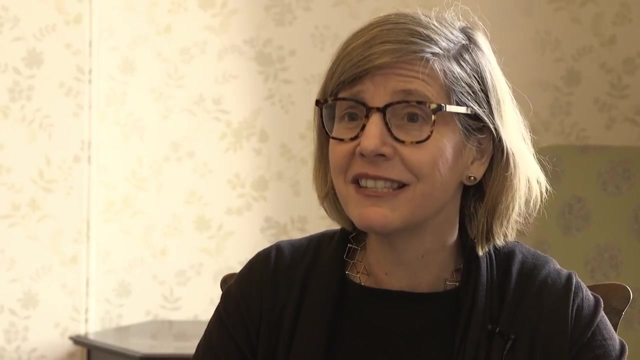 as the law of environmental problems. Some problems are going to be very local contaminated land. Others are going to be global climate change. A common feature of environmental problems is that they are both physically complex and socially complex. They're physically complex because they involve ecosystems. If we put fertilizer on agricultural land and it runs off into rivers. a whole range of implications might happen for the natural environment and also for human health, But they're also socially complex. Environmental problems are often caused by a range of different people not intending to harm the environment, but 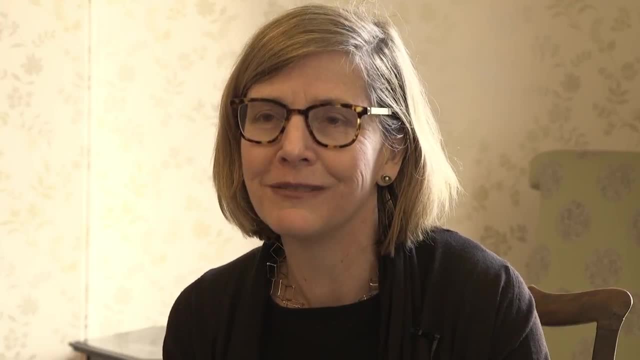 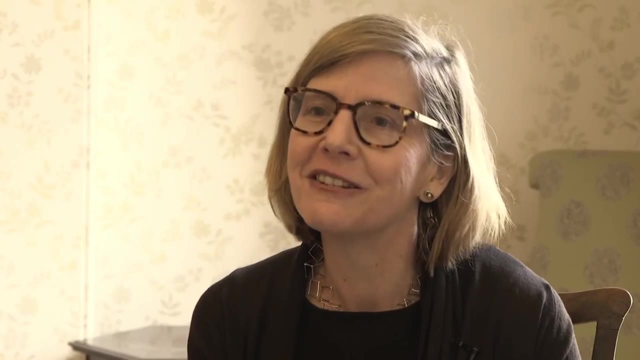 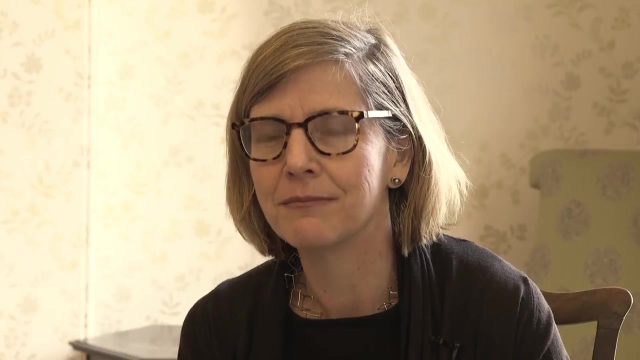 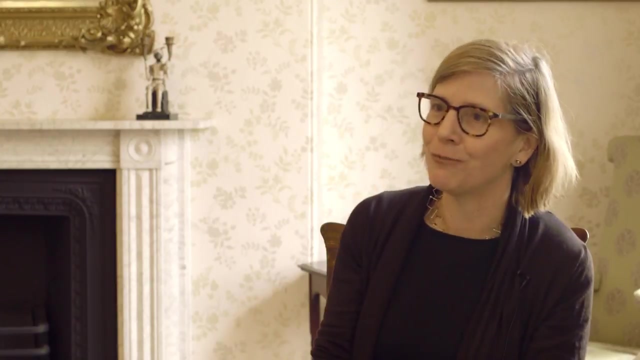 each of their actions contributing to an environmental problem. Nation states play a significant role in environmental law, and that's because they have the authority and the capacity to develop collective responses in relation to these problems. Modern environmental law really has its roots in the 1960s, and it wasn't just a response to environmental problems, It was also 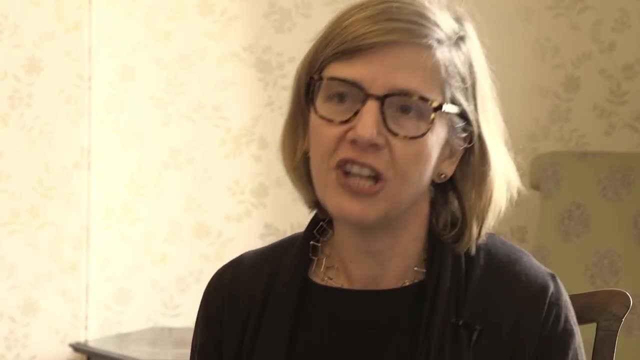 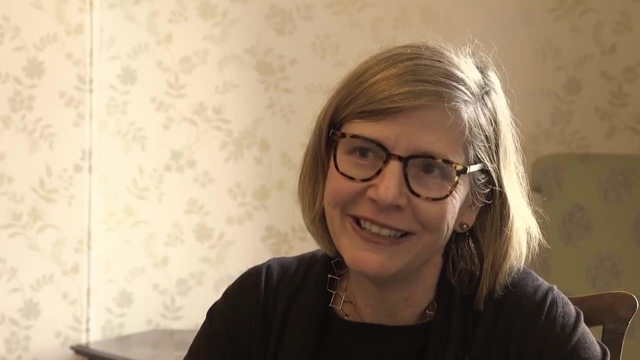 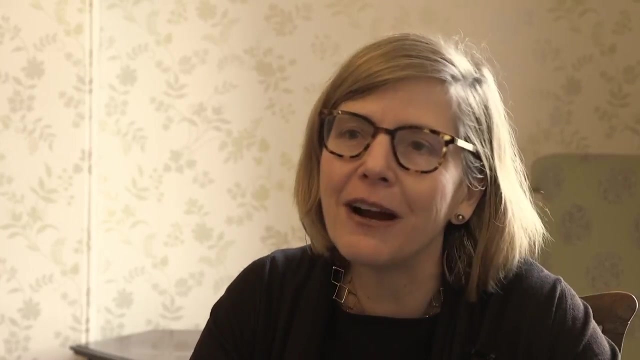 part of a commitment to make societies more just, more fair and more democratic. Environmental law is not a magic wand. It's not a case of passing a piece of legislation, signing a treaty or a court deciding a case and an environmental problem disappears. 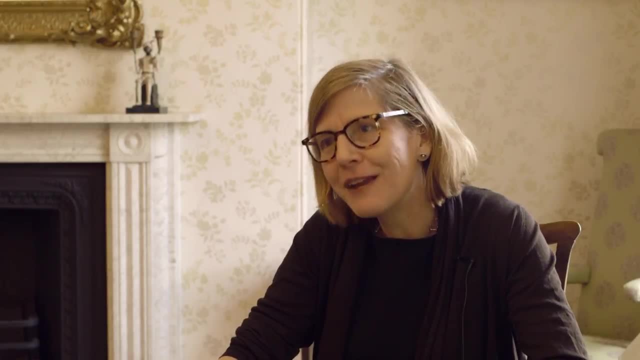 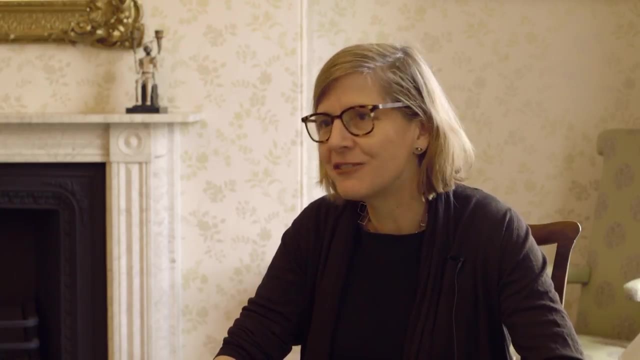 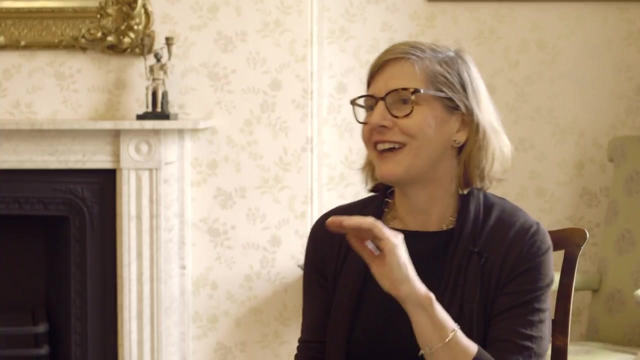 What is required is the creation of legal frameworks which ensure the ongoing management of an environmental problem in as fair and just a way as possible. Environmental law is very technically complex. If you look at a textbook on the environmental law of any country, it's big. 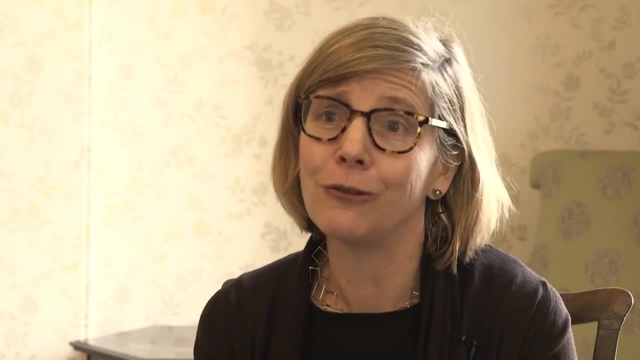 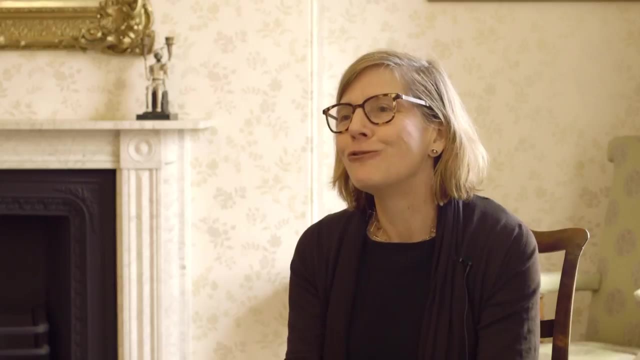 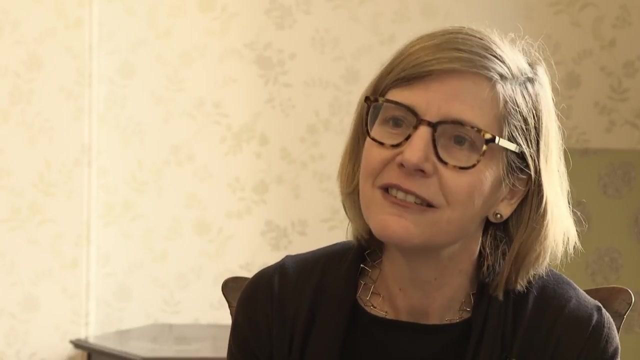 it's thick. Environmental lawyers need to know a lot of law and they know how to apply it. with nuance and sophistication, Environmental law has required the expansion of the legal imagination. That's because a lot of law hasn't developed with the environment and these type of collective 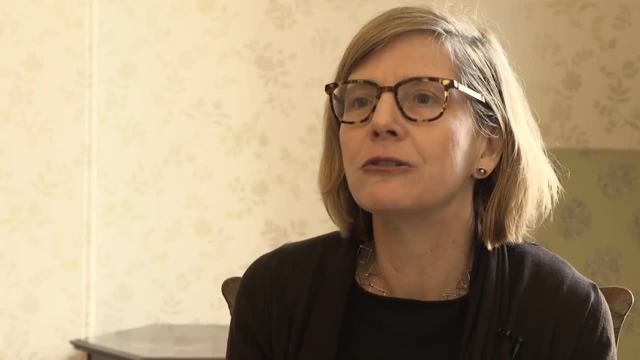 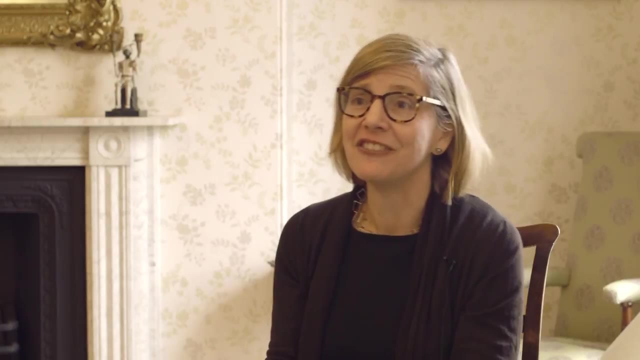 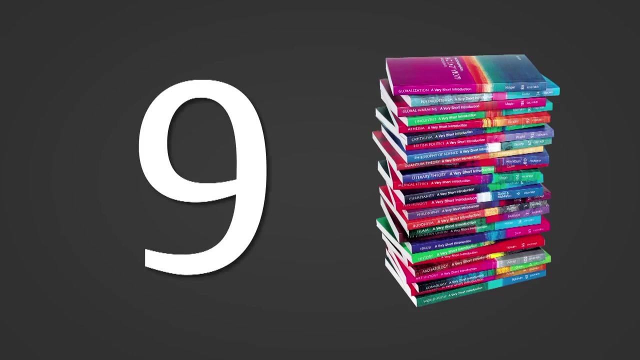 action problems in mind, And so, with the development of environmental law, we've had to think about different types of legal obligations In countries such as India, and there have been legal developments where the legal rights of rivers have been recognised, An important theme in environmental law is environmental justice. But environmental justice means many different things. It might mean justice between nations, justice across generations, justice within local communities, or even a form of justice that takes the rights of the earth into account. Environmental law is often controversial. We might debate whether there's an environmental problem.